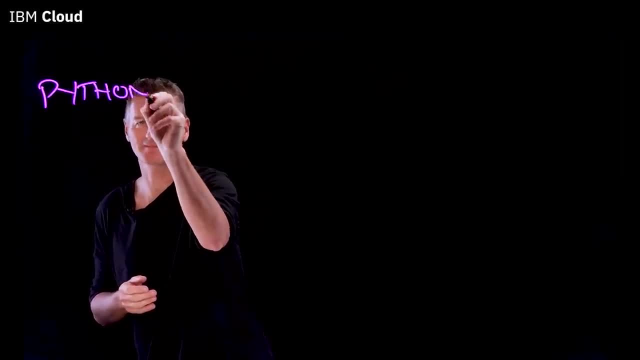 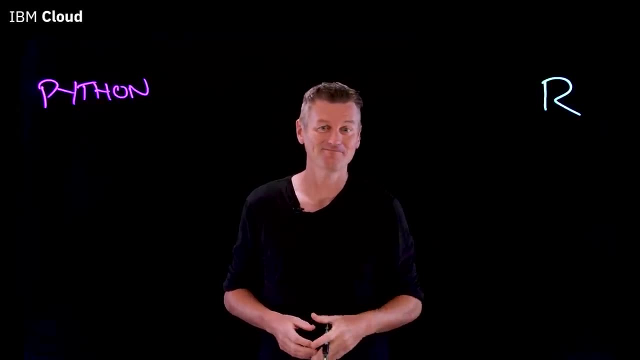 Python is an open-source programming language commonly used in data science, as is R. Which one should you be using At this point? you might be expecting a fence-sitting- well, it depends, kind of answer. but no, I'm going to tell you exactly which one to pick. 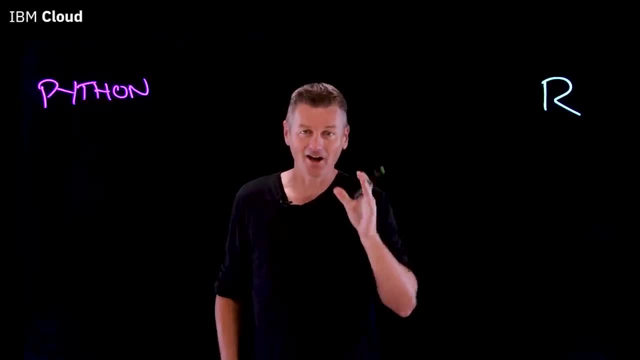 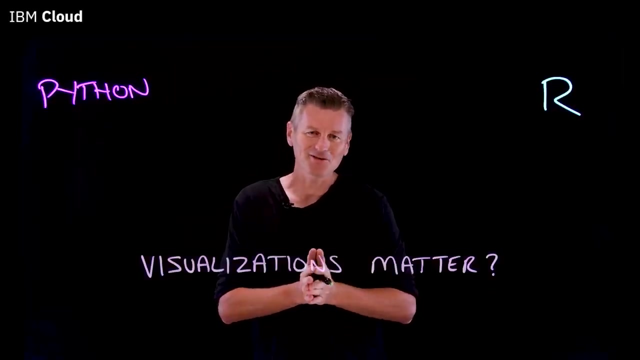 right now. So here goes: I ask you a question and based on your answer, you'll know which language to go for. Ready, Okay. so do you have much in the way of programming experience? None use R. Some go for Python, Lots R. again, I'll explain. Okay. question two: Do you care about? 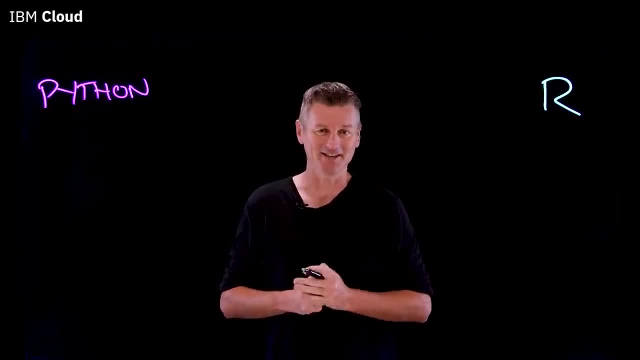 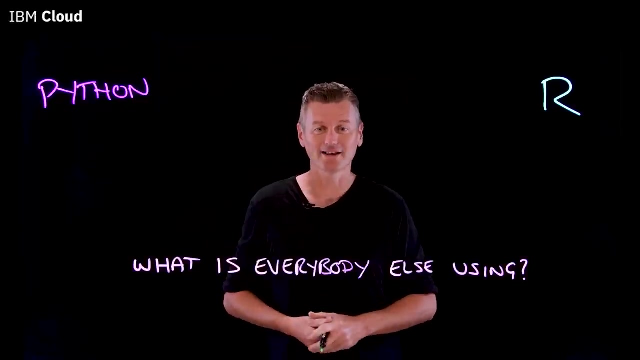 awesome-looking visualizations and graphics. If yes, go with R. What about the problem you're trying to solve? Machine learning stuff? Go with Python. Statistical learning R is your best bet. And finally, what do most of your colleagues use? 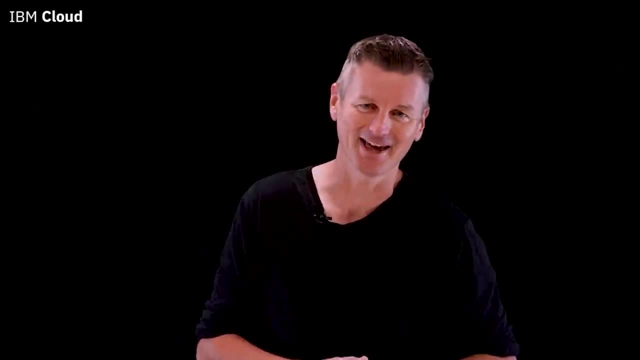 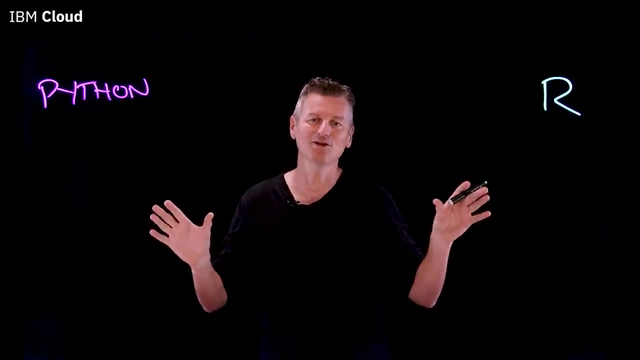 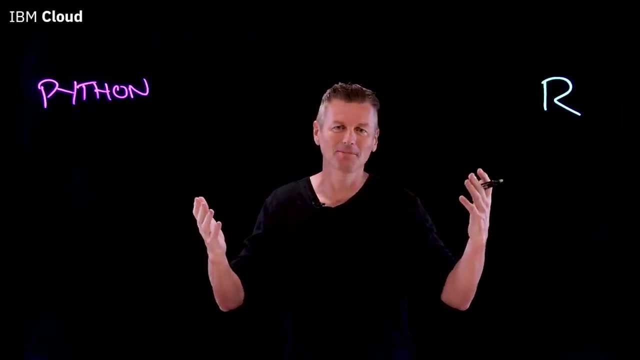 Use that Glad to get that off of my chest Now. we could all just finish here and go about our day, but I'd like to explain a little bit more about what these two languages are and how they're best put to use, because increasingly the question isn't which to choose, but how to make the best. 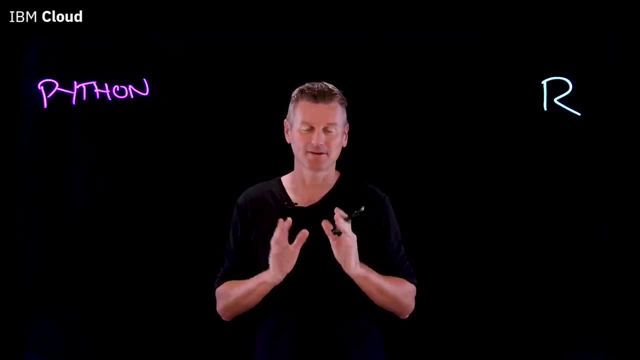 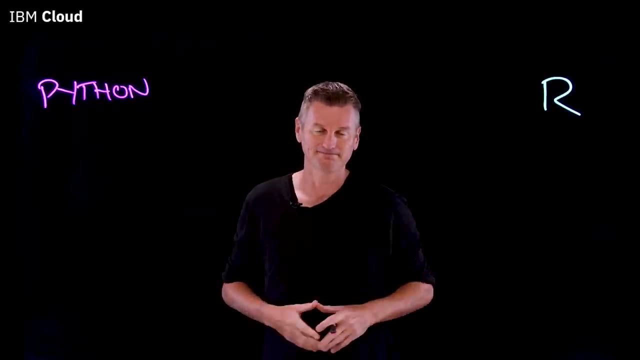 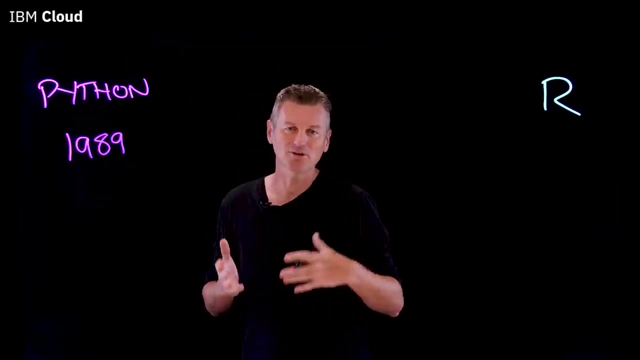 use of both programming languages for your specific use cases. So let's start with the slightly older of the two, which is Python. Now, Python was released in 1989, and it's a general purpose object-oriented programming language that emphasizes code readability through its 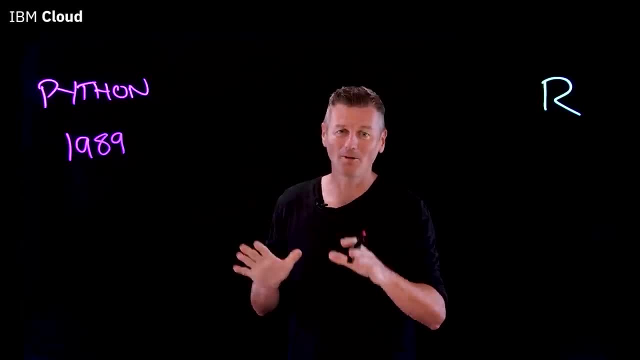 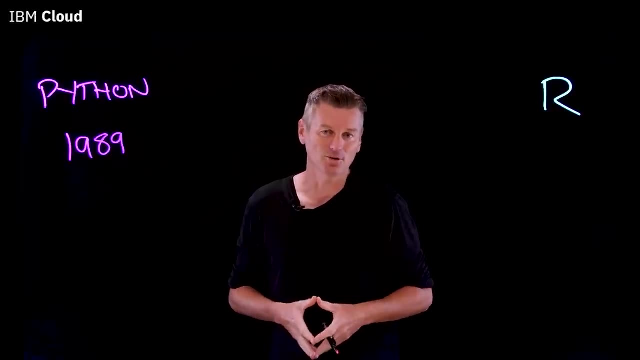 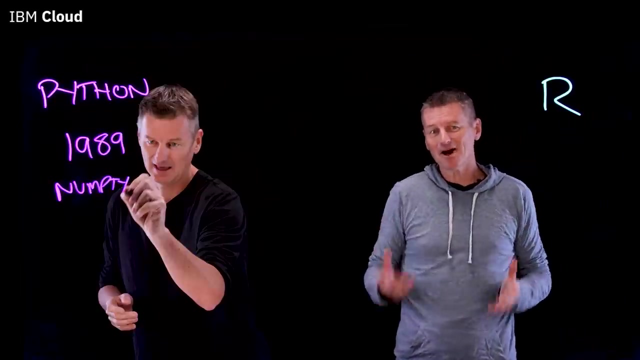 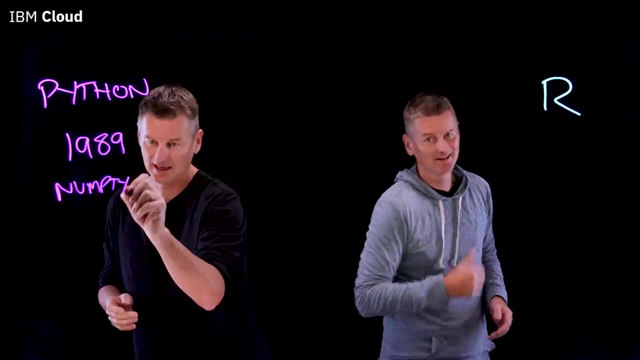 generous use of white space and it's super popular, just behind Java and C in popularity. In fact, there are some awesome libraries that support data science tasks. So, for example, we have numpty. It's actually numpy numpty. that's British slang for an idiot, numpty and numpty is used for 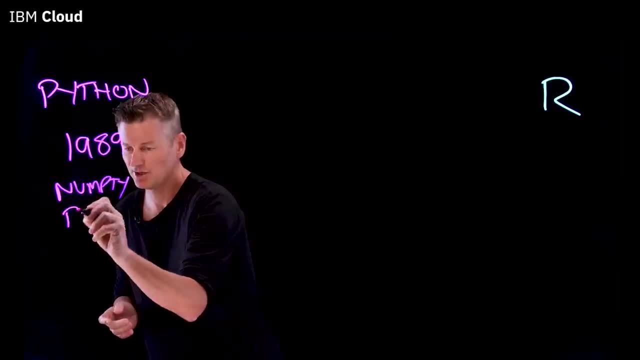 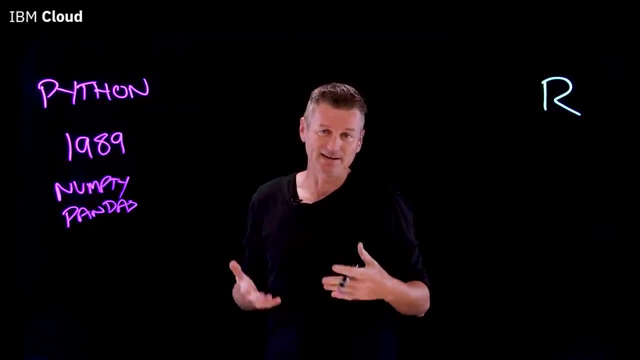 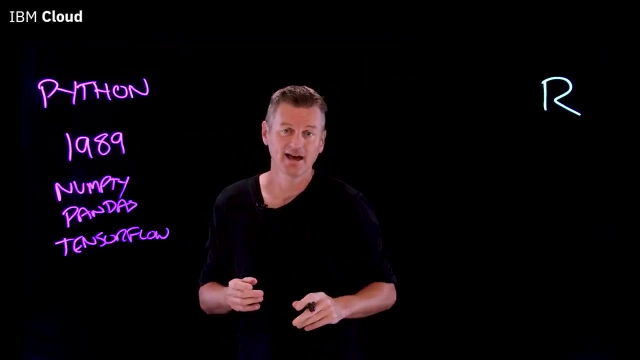 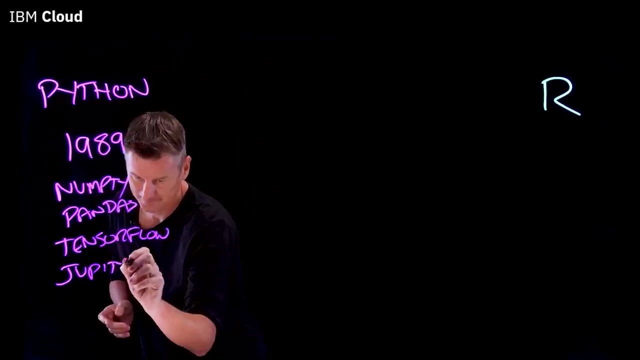 large dimensional arrays, and then for data manipulation we have pandas. There are also specialized tools for deep learning, so you can use things like TensorFlow, And you'll often find yourself working with Python in Jupyter Notebooks as your IDE. 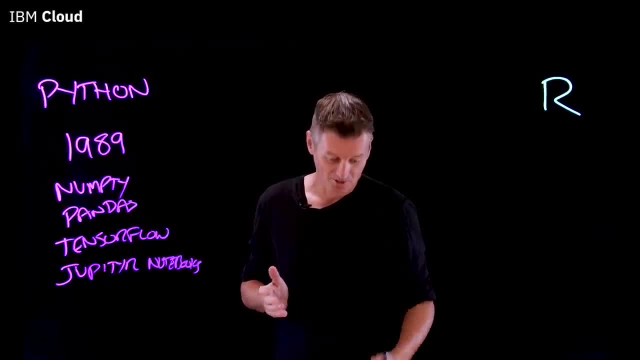 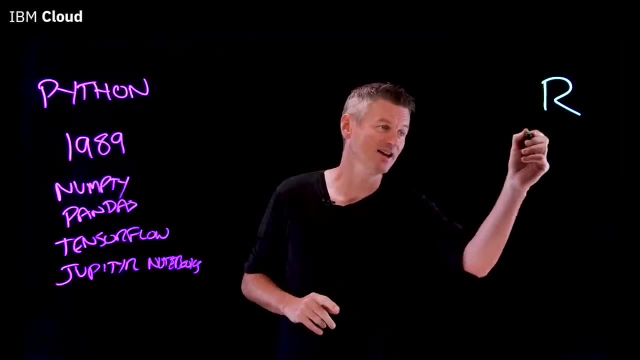 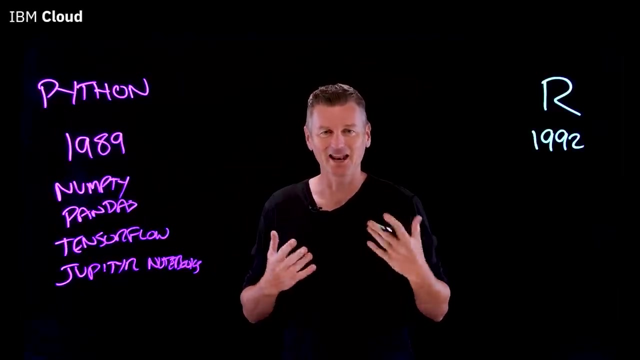 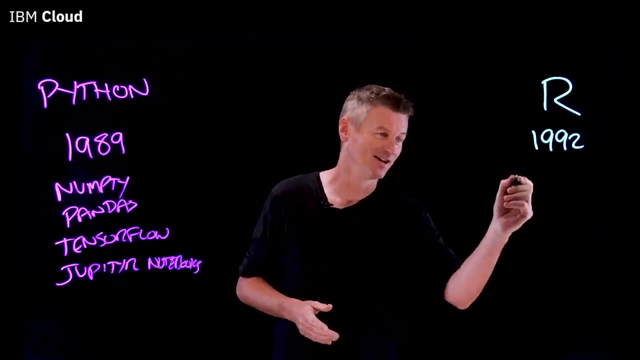 Now let's compare that to R, which is optimized for statistical analysis and data visualization. So it was developed just a little later, in 1992, and it has a rich ecosystem with complex data models and elegant tools for data reporting. There are thousands of packages available via the comprehensive R archive network, otherwise known as CRAN. 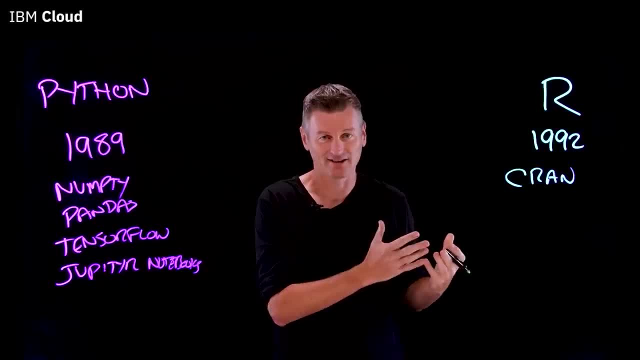 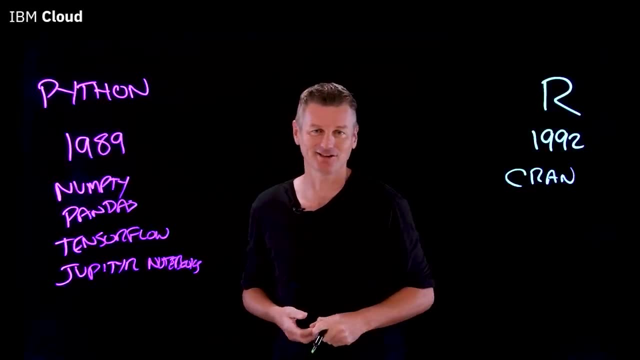 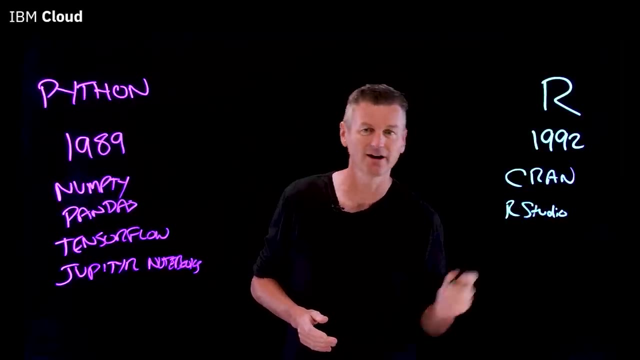 And these things are for deep learning. Now, R provides a broad variety of libraries and tools for things like cleansing data, creating visualizations and training deep learning algorithms, And R is commonly used with R Studio, which is an integrated development environment for simplified statistical analysis, visualization and reporting. 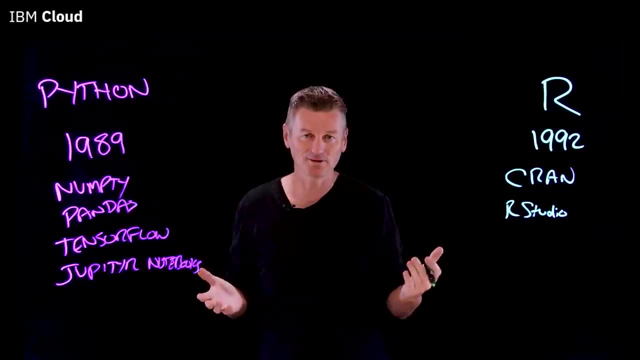 So both R and Python are open source and are supported by large communities continuously extending their libraries and tools. Really, the biggest differentiator is how they are used, and R, as I've mentioned, is mainly used for statistical analysis, while Python provides a more general approach to data wrangling. 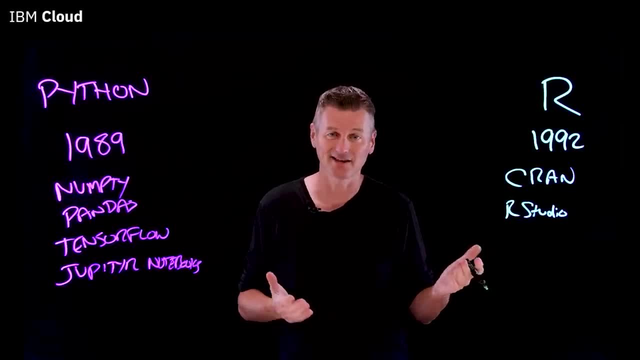 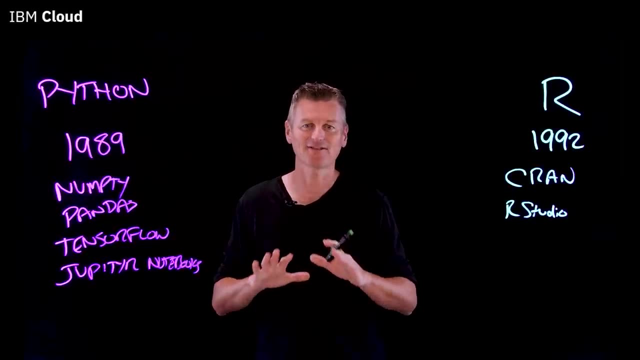 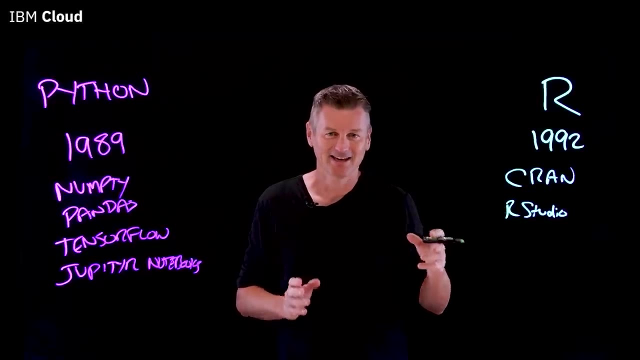 You might use R for customer behavior analysis and then you might use Python to build a facial recognition application. Now, right up front, I said: if you have no programming experience, or quite a lot of programming experience, R was the better bet. Now, if you have a computer or a laptop and you're not comfortable somewhere in between, then Python is easier to pick up. 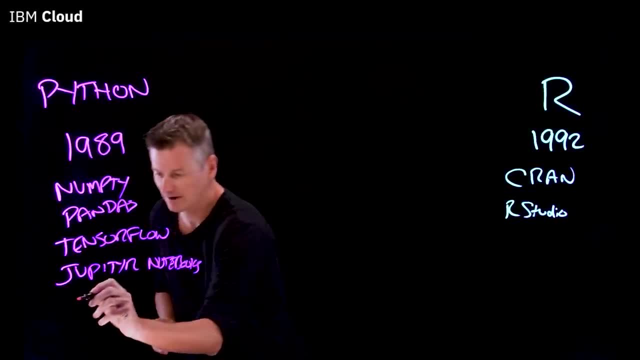 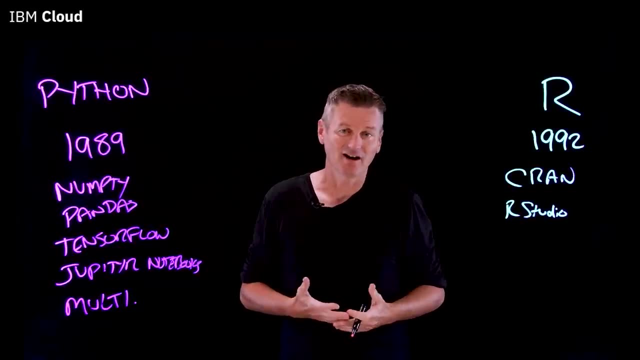 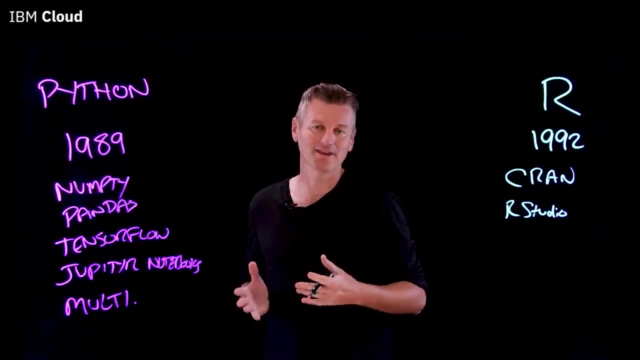 But how can that be? Well, Python is multi-purpose. It's considered a multi-purpose language, Much like C++ and Java R, and it has a readable syntax that's easy to learn. It's considered a good language for beginner programmers. 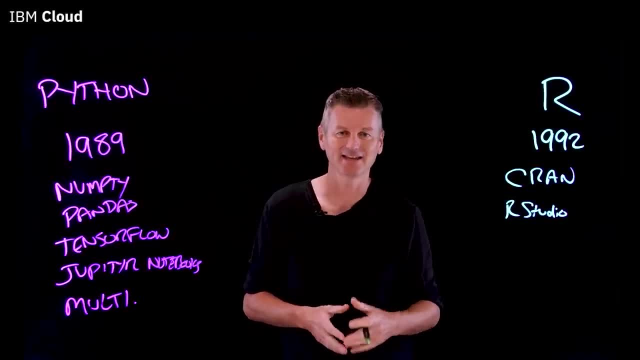 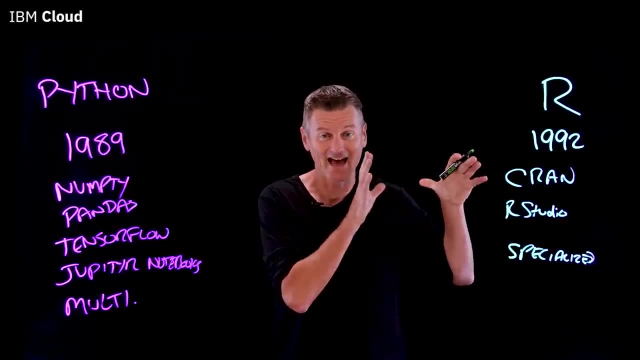 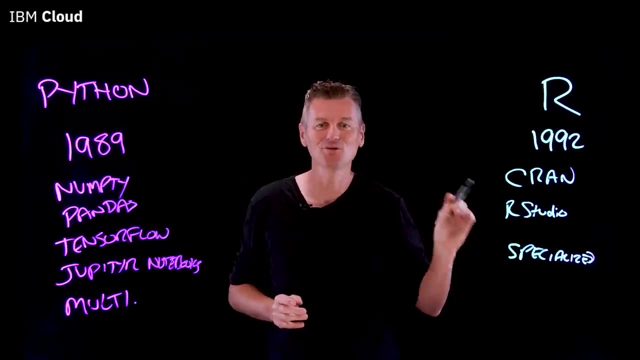 or those with experience in similar languages, built by statisticians and leans heavily into statistical models and specialised analytics. Now novices can be running data analysis tasks within minutes with just a few lines of code using R, but the complexity of advanced functionality in R makes it more difficult. 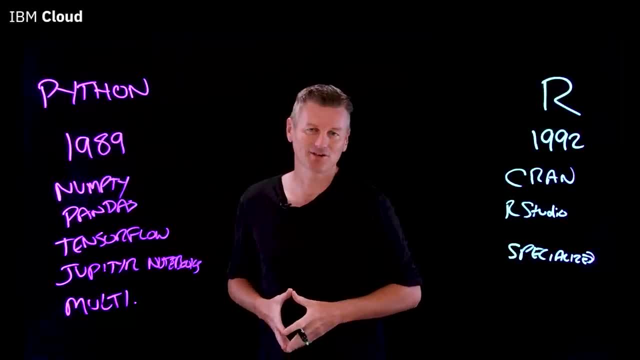 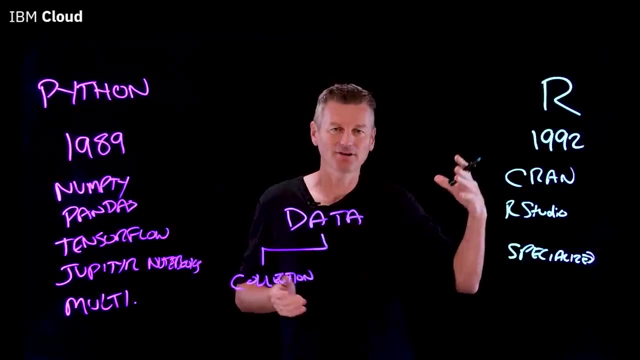 to develop expertise. Now a few other considerations to keep in mind, and they all relate specifically to data. Now, when it comes to data collection, so actually gathering the data in the first place, Python supports all kinds of data formats, from comma separated value files or CSV files. 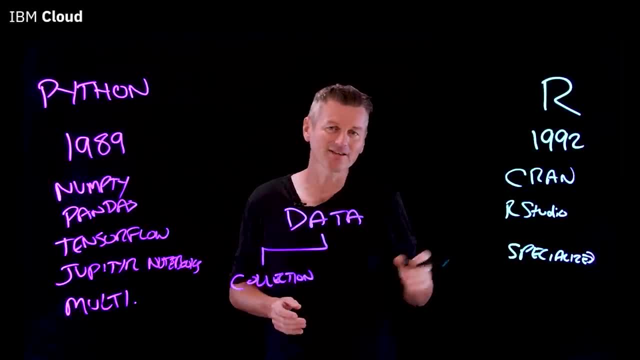 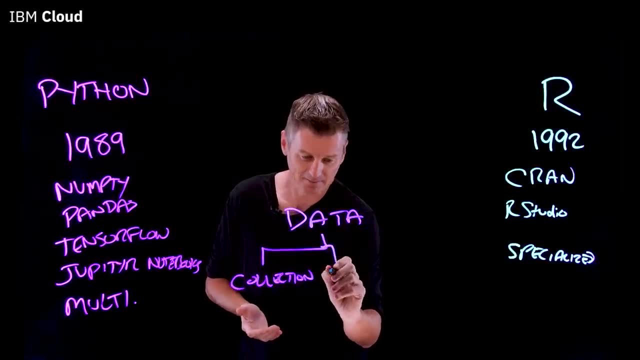 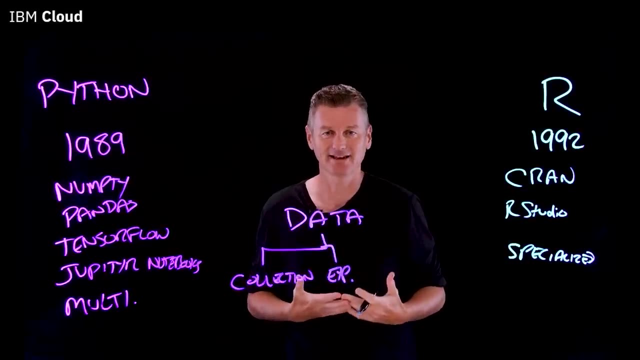 to JSON sourced from the web. In contrast, R is designed for data analysts to import data from things like Excel and Txt files. Now for data exploration. then you can use the pandas library to filter, sort and display data In a matter of seconds if you use Python. and R, in the other hand, is optimised for statistical 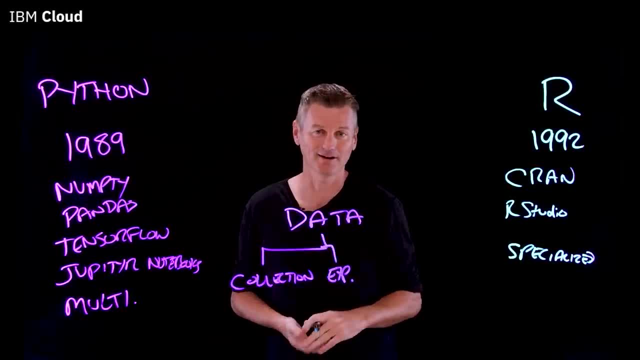 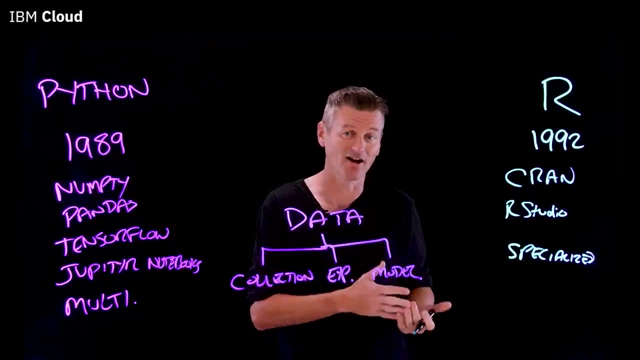 analysis So you can build probability distributions or apply different statistical models. And then, finally, data modeling has some differences too. Python has libraries for data modelling. like numpty in R, You'll sometimes run fascinating認為. you'll sometimes have to rely on packages outside of R's core functionality. 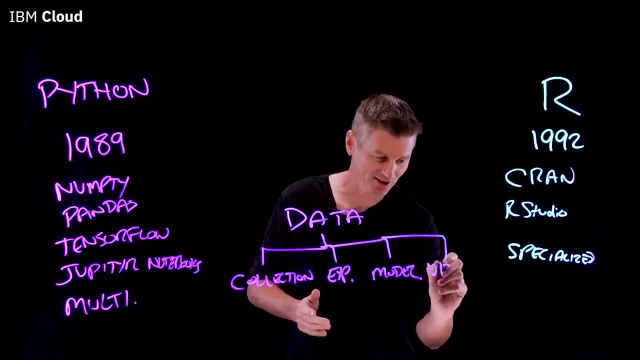 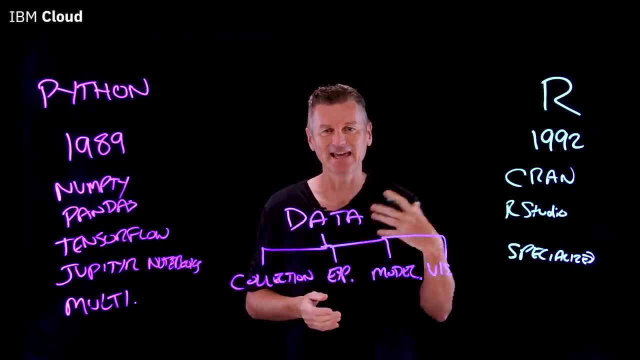 Did I see? Finally, there's one more, and that's visualization. And with visualization, R has the clear edge, with a base graphics module allowing you to easily create basic charts and plots, And you can use ggplot2 for more advanced plots. 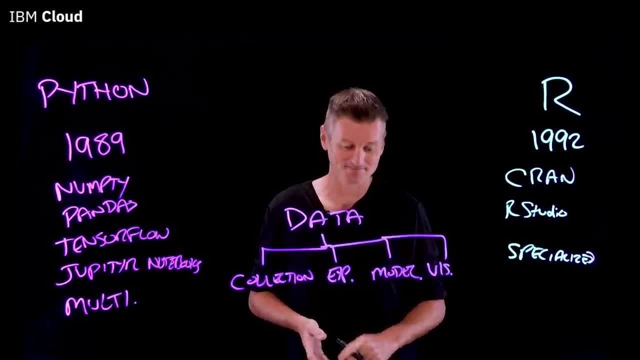 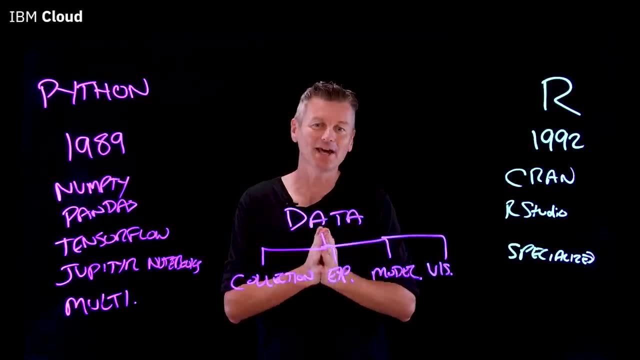 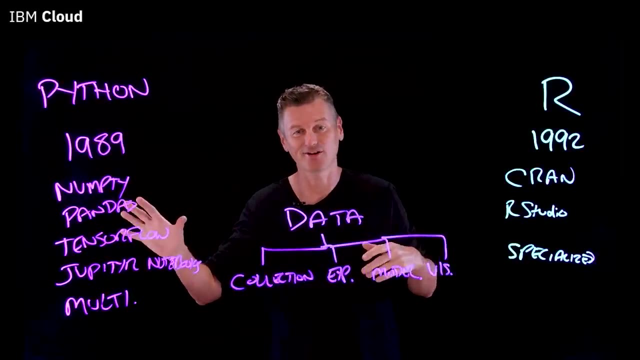 such as complex scatter plots with regression lines. R and Python have their strengths, but in truth, most organizations use a combination of both languages. You might conduct early stage data analysis and exploration in R and then switch to Python when it's time to ship some data products. 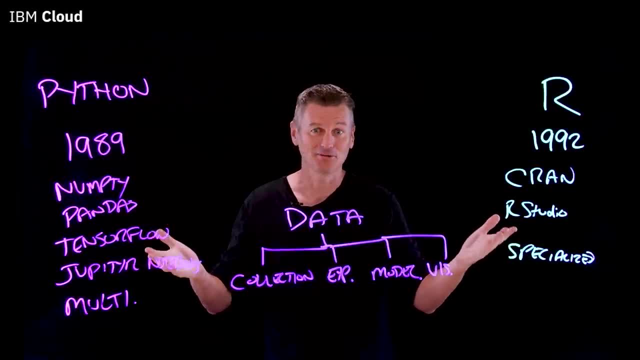 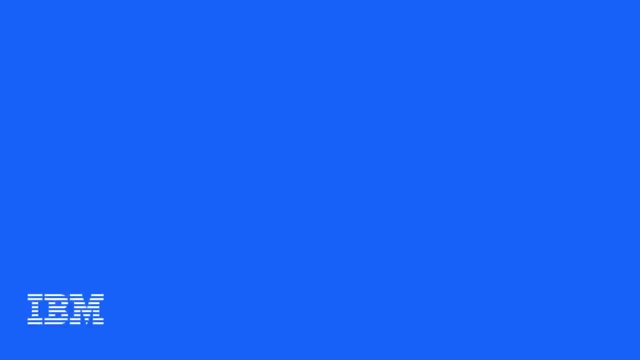 So which should you use Both? You're probably going to use a bit of both, And if you want to see more videos like this in the future, please like and subscribe. Thanks for watching.